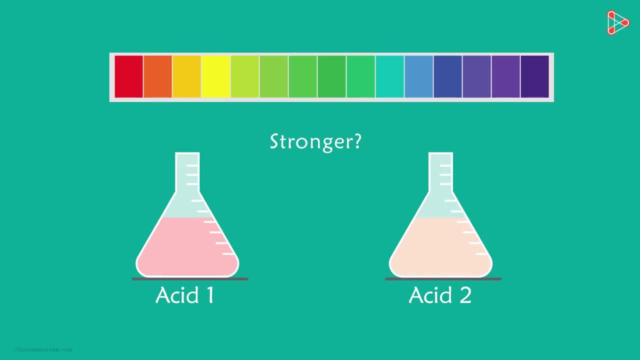 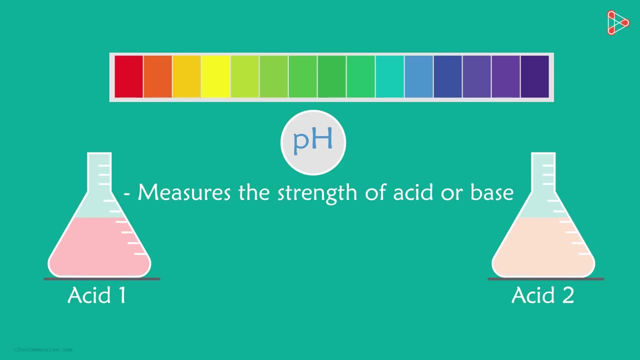 How can we judge how strong an acid or a base is? And that's what pH helps us with. It gives us the measure of the strength of acids or bases. How does it do that? The pH takes into account the concentration of H plus ions in the solution. 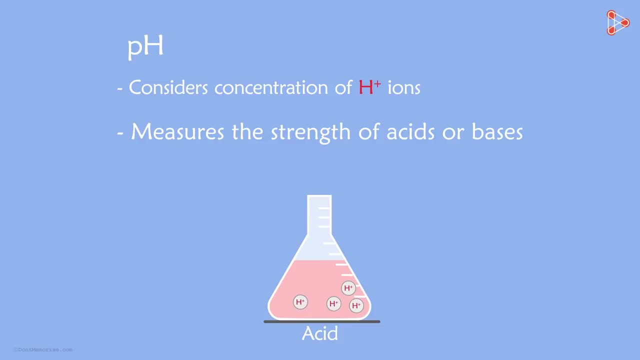 Yes, the pH measures the strength of acids, But you'd probably be thinking that if pH only considers the concentration of H plus ions, how can it tell us how strong a base is? Remember, bases also contain H plus ions, Just that the concentration of H plus ions is far lower than that of the concentration of OH minus ions. 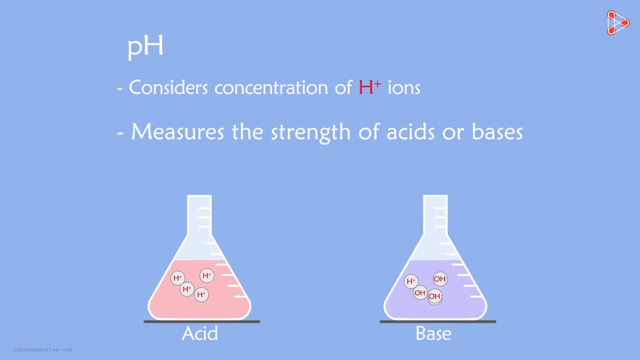 so low that they are generally ignored. So to know how strong an acid or a base is, we have the concept of a pH, And it ranges from 0 to 14.. 0 being very acidic and 14 being very basic or alkaline. 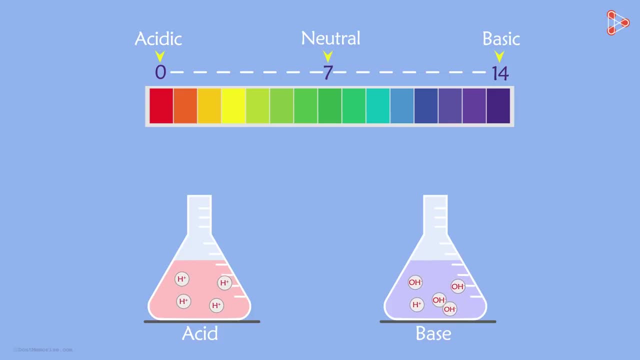 And the pH of a neutral solution right here in the middle is 7.. Understand that the pH is just a number which tells us how acidic or basic a solution is. More the concentration of the hydrogen ion, lesser will be the pH value. Yes, understand this well. 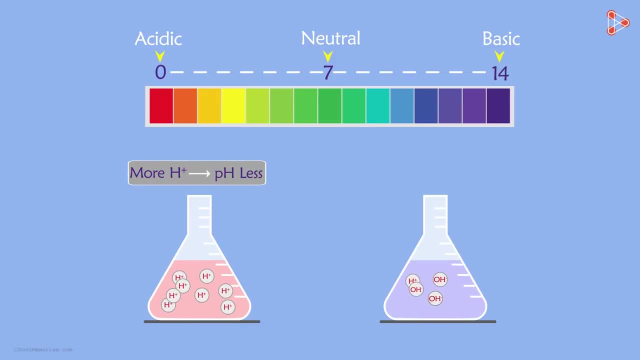 More the concentration of the hydrogen ion, lesser will be the pH value. Now, if you look at the scale, as we go towards the left, the pH value is decreasing, Which means that if we go leftwards on this scale, the H plus ion concentration increases. 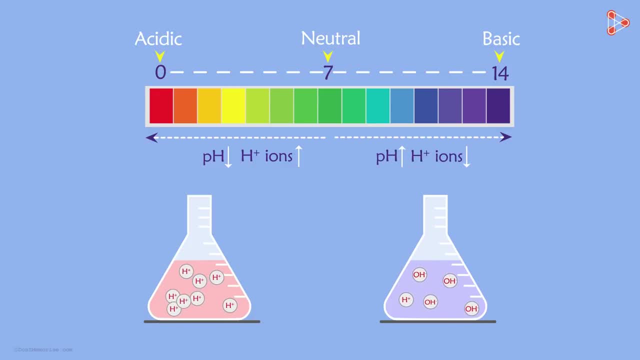 And as we go rightwards the H plus ion concentration reduces. And we know that higher H plus ion concentration implies that the solution is more acidic. So the acidic nature increases as we go towards the left And as basic solutions have lower concentration of H plus ions. 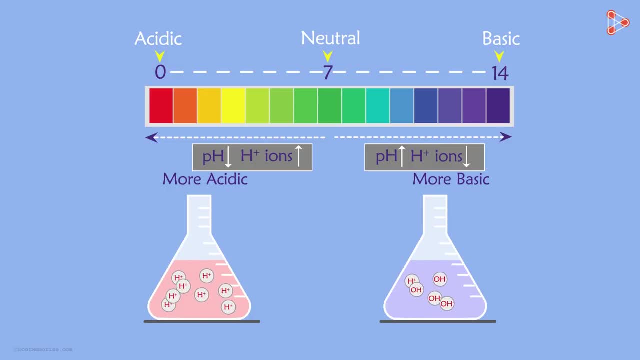 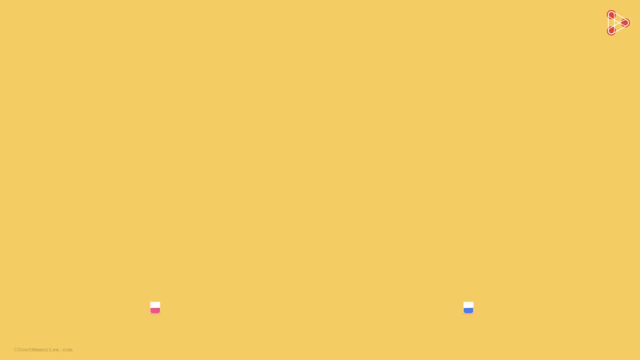 the basic nature increases as we go towards the right. So this pH scale is a very general way to understand how strong an acid or a base is. Let's take a very basic test to check if you've understood the concept of pH scale. I have two solutions: A and B.